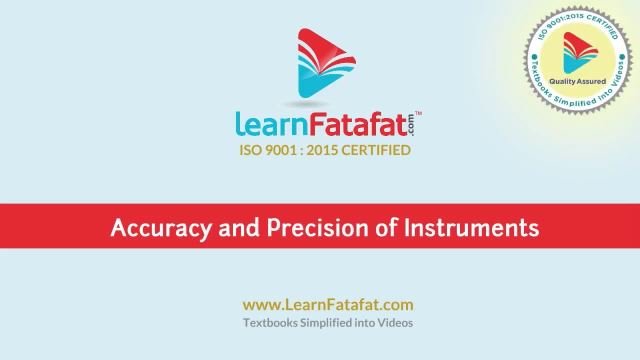 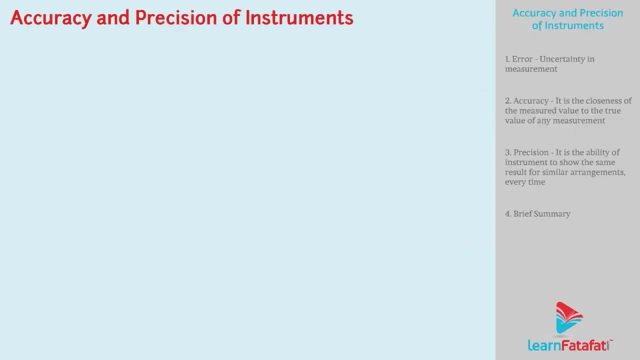 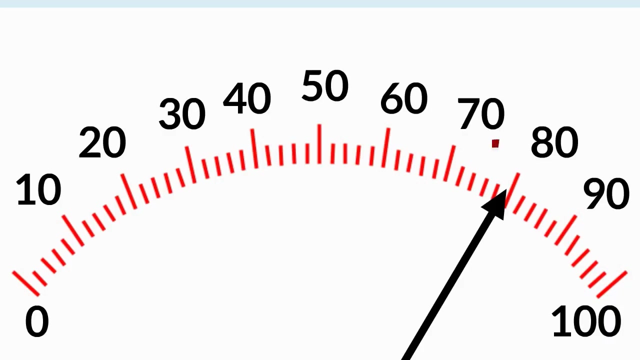 Accuracy and Precision of Instruments. Dear students, Measurement is integral part of physics. In any experiment, there is need of measurement. However, the result of every measurement may have certain uncertainty. Let's discuss this with the help of an example. What if someone tells you: 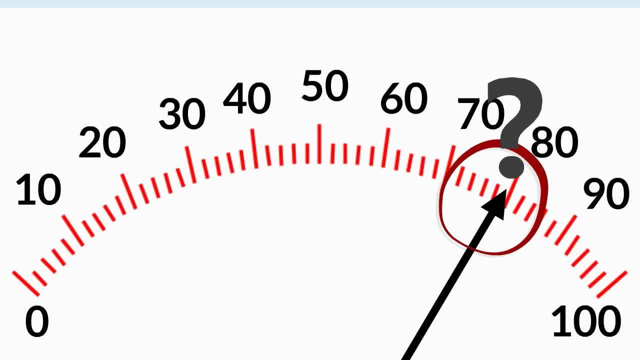 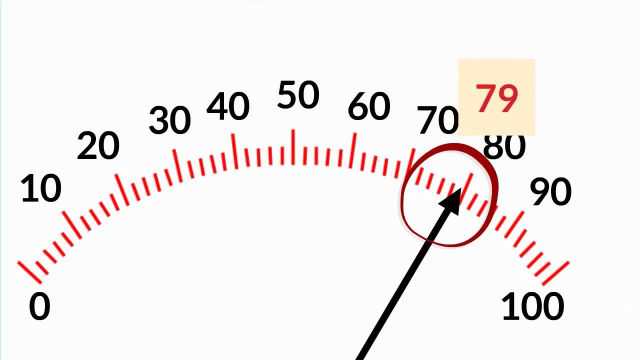 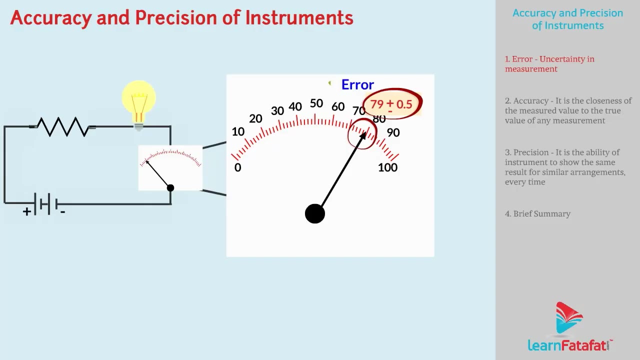 that identify the reading in the given figure? Can you? Even if you decide any value, still the reading has certain uncertainty. So such type of uncertainty is called error, As we know the term error. Now let us understand accuracy and precision. 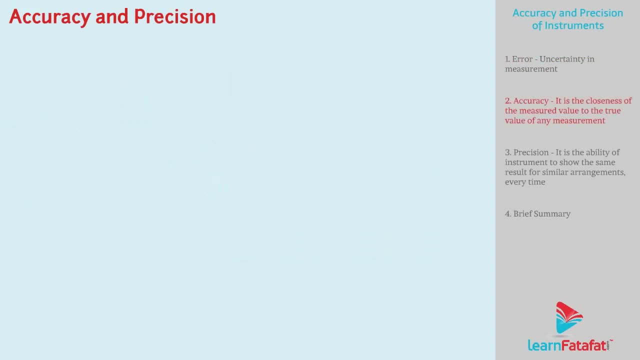 Are they same? No, Let's distinguish between them with the help of an example. A resistor is designed to provide the resistance of 100 ohms. We take two multimeters and measure the resistance separately. If the reading is 100.1 ohm in the first multimeter, 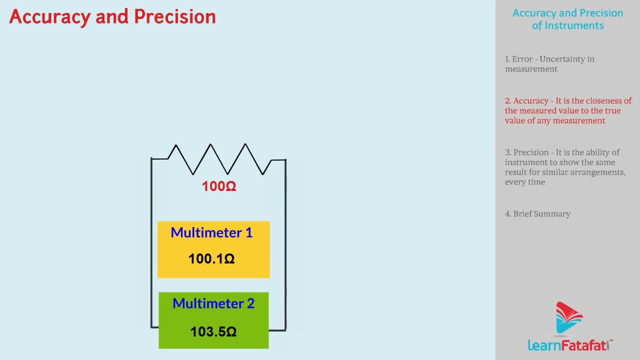 and 103.5 in second multimeter. we say that first multimeter shows accurate reading. So what accuracy is? Accuracy can be defined as the closeness of the measured value to the true value of any measurement. Consider the same example of measuring the distance of 100 ohm resistor.